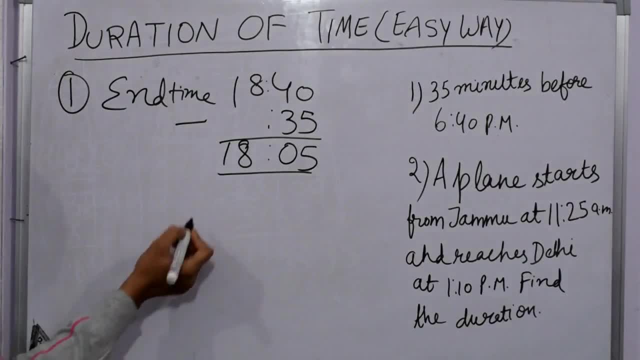 This is our answer: 18.05, or you can say 6.05 pm. Now the second sum is: a plane starts from Jammu at 11.25 am and reaches Delhi at 1.10 pm. In this sum we have starting time and ending time. 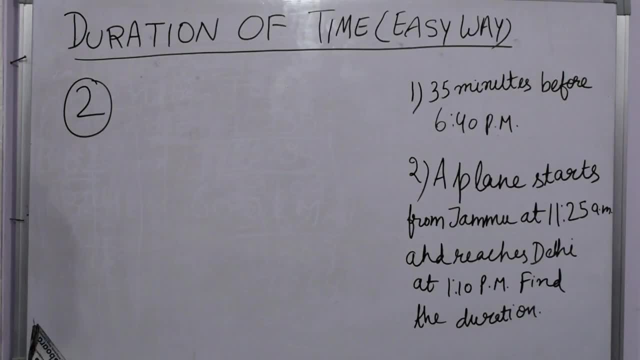 We have to find out only duration. Convert each and every time. Convert it every time into 24 hour clock. Reaches Delhi at 1.10 pm. Convert it into 24 hour clock. We got 13.10.. Starts at 11.25 am. 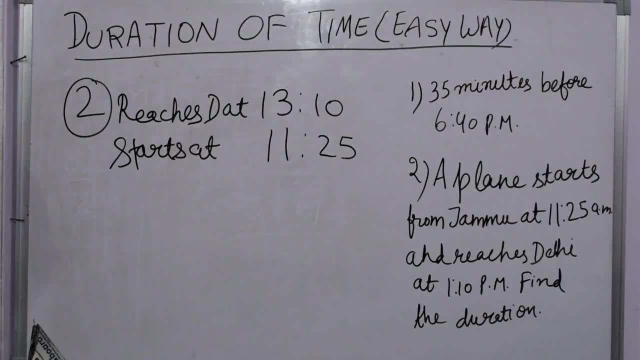 So 24 hour clock, we will write out it as 11.25.. Now, subtract, We got 185.. Now, in this case, where we got minutes more than 60. Equal to 0 more than 60. And we are subtracting here. 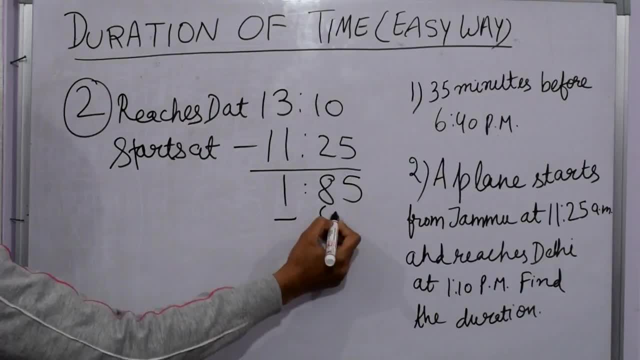 We just subtract 14 from the minutes side, We got 5. And this is our answer: 1 hour 45 minutes. This answer is in hours and minutes Because we have to find out duration And the previous one is in pm. 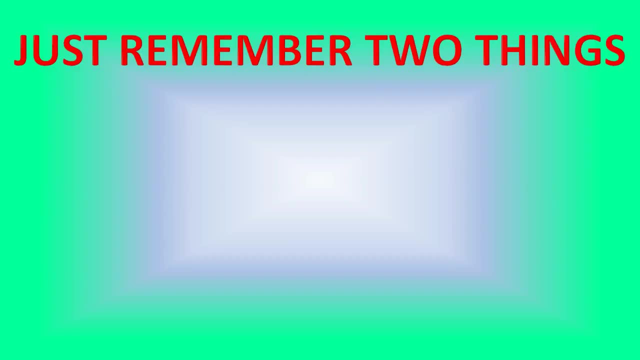 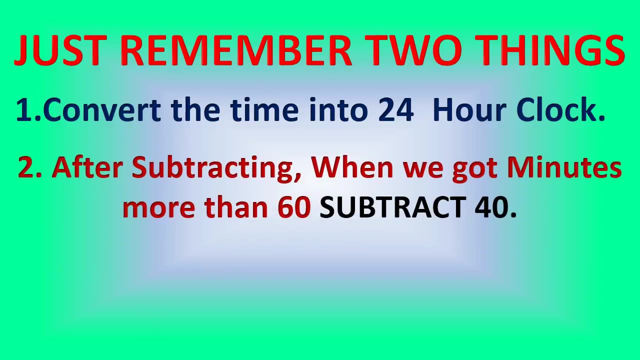 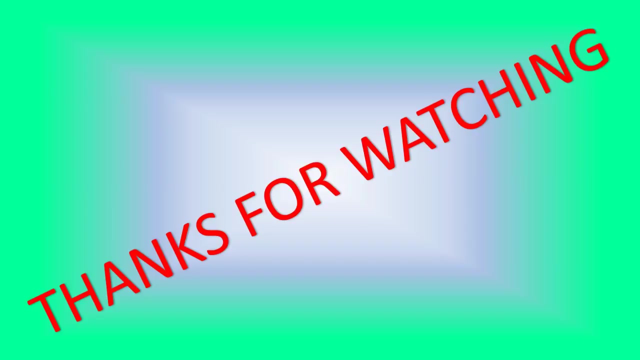 Because we have to find out starting time. Just remember two things: Convert the time into 24 hour clock And, after subtracting, when we got minutes more than 60. Subtract 40.. Thanks for watching And don't forget to watch our next video on finishing of time. 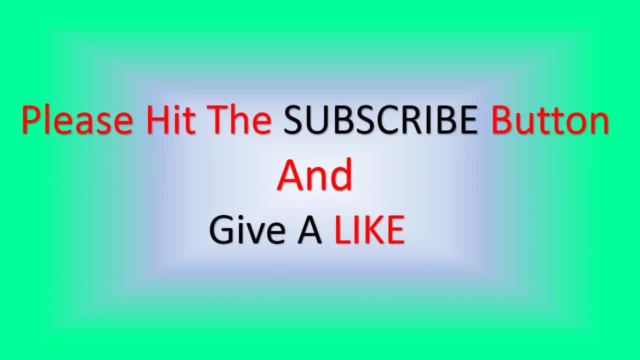 If you like the video, please hit the subscribe button and give a like, And don't forget to share. Thank you.